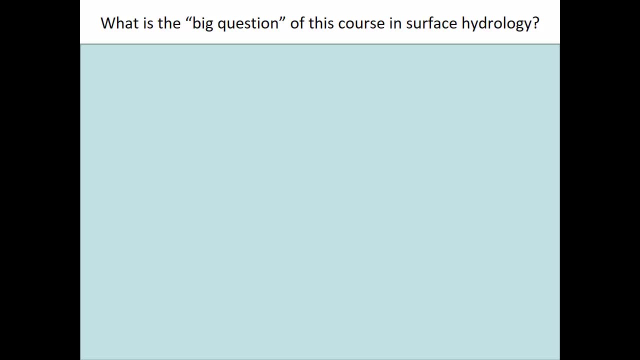 There could be a course out there where the big question is: how much does a force deflect the material? Or there could be a course where the big question is: how does time affect the value of money? So that's an illustration of the big question of 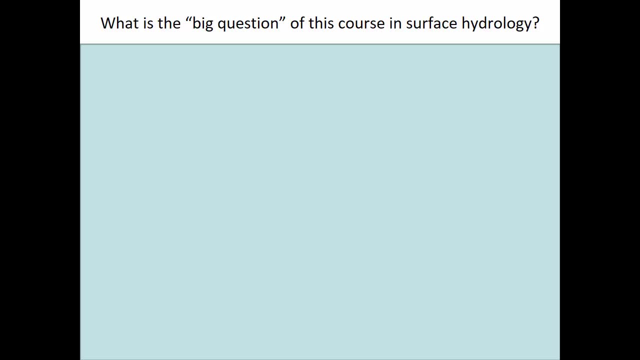 engineering, cost analysis and economy, But what do you think in a course about surface hydrology? what's the big question? I'll give you just another minute to think about it, All right? Anybody interested to share what they wrote down as the big question for the? 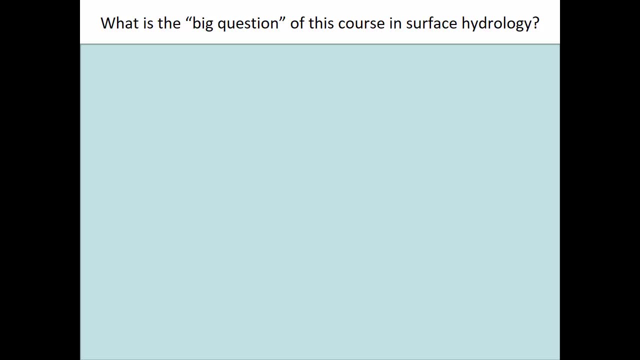 course. What did you say, Jeffrey? Why does the water pack impact the water? Why does the water pack impact the water? Why does the water pack impact the water? Okay, good, Why does the water act this way? That's an excellent stab at it. Anybody else? 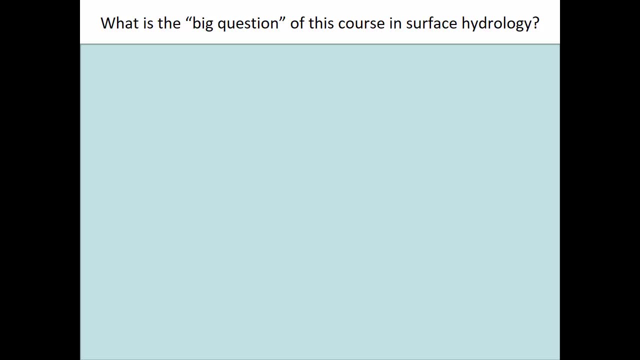 have a go a different direction. Yes, How much water is present on the surface of an area and how does it affect its quantity? Good, So, the amount of water and what's the effect that that water has? Excellent, Well done, All right. So here's how I put it For an area of interest. so we're talking about 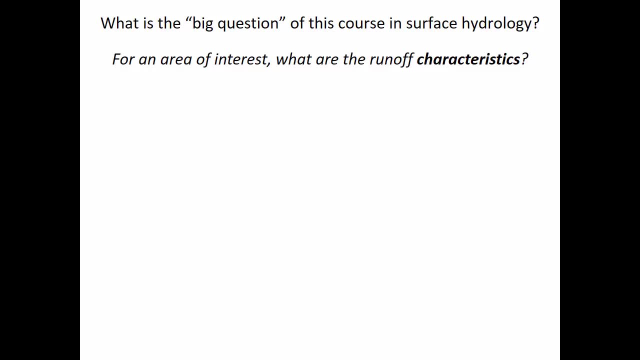 a certain area. What are the runoff characteristics? Now, to explain why I put it that way, what I have to do is draw the distinction between hydrology- Oh, that marker's done- Hydrology and hydraulics. Okay, Now hydraulics, which some of you have done, some of you are doing later this afternoon. 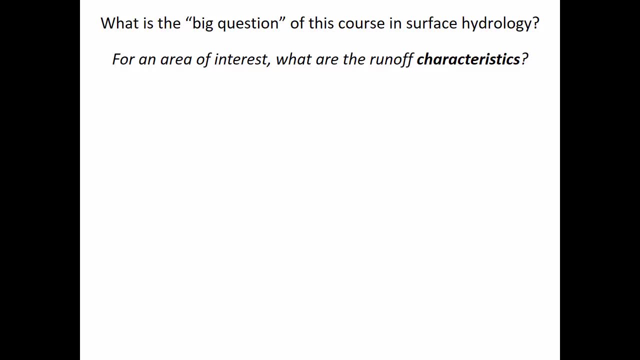 is basically saying, for a certain flow rate, how big of a pipe is needed. So that's the diameter of the pipe. You know, if we're talking about water that is moving through the environment, so open channel flow, For a certain flow rate, how big of a pipe is needed? Well, the diameter. 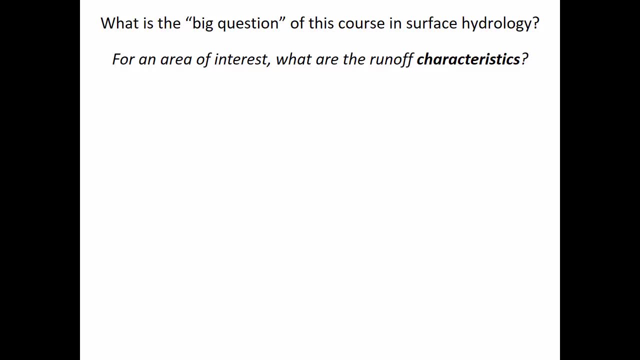 of the pipe. How big does the pipe need to be? That's what hydraulics answers. So what hydrology answers what I said in words here. for an area of interest, what are the runoff characteristics? And so what we're doing is we're getting Q based on area surface. 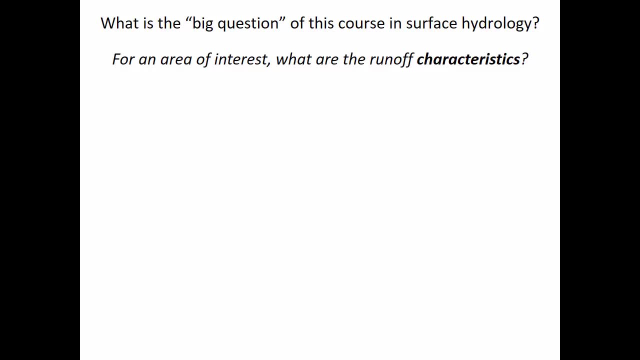 characteristics: rainfall, evaporation- So we're getting Q based on the flow rate. So there's a whole lot of things that determine when it rains how much water is actually getting to a certain place. So have you ever driven down Fifth Avenue on a rainy day? What did? 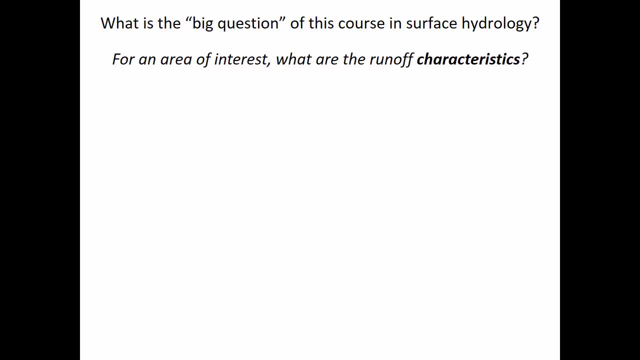 you notice, as you drove down Fifth Avenue on a rainy day, That on the side the water pools up. a whole lot of water. It does, Yeah, it pools a lot, And if it's an extremely rainy day, is that like four? 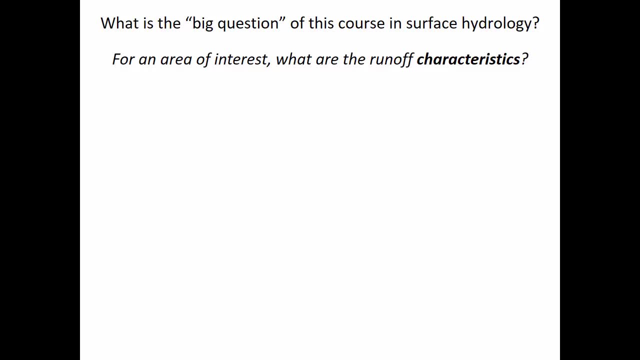 lanes Like that. The outer two lanes are no good and you can only drive in the center two lanes And so it really slows down traffic. So hydrology gives the hydraulic engineer the information that the hydraulic engineer needs to size the pipe. The hydraulic engineer just takes. 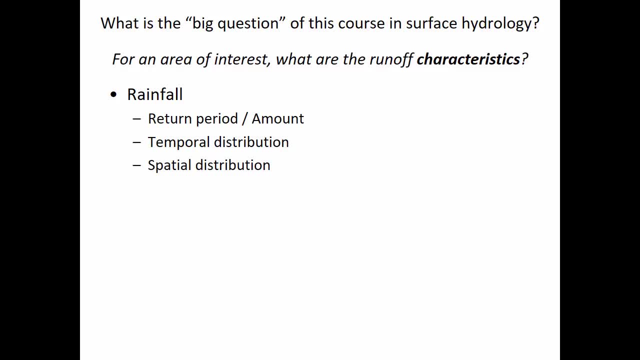 the defined flow rate and figures out how big the pipe needs to be. So what the hydrologist does is: the hydrologist looks at how much is it going to rain? What is the area like Like? is the water going to be a lot of water? Is it going to be a lot of water? Is it going? 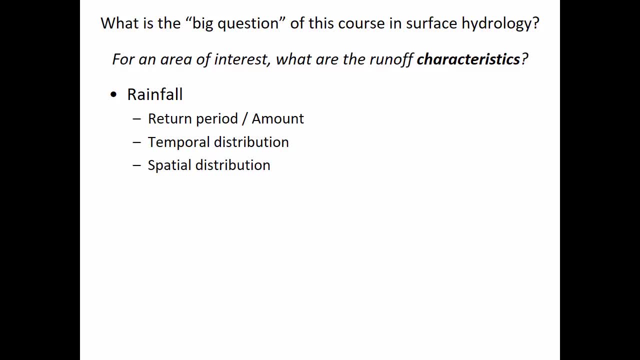 to get down into the soil versus is it going to run over the surface, And so the hydrologist tells the hydraulic engineer how much water to expect. So here are all the inputs to that. We have to understand the characteristics of rainfall, Not only how much rainfall there's going to be, like I'm sure you've heard on the news. 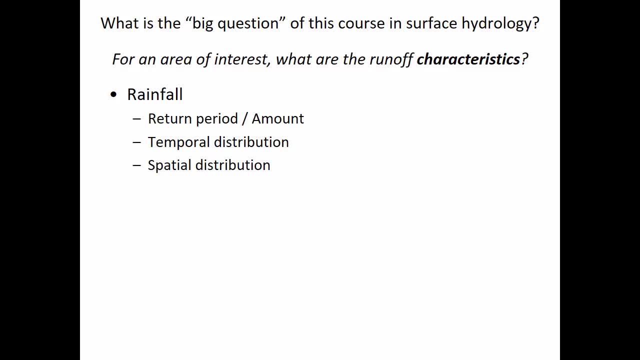 they'll say: well, it rained 0.7 inches today. Well, the amount is important, but the timing of the rainfall matters. The timing of the rainfall is just as important, maybe even more important, than the absolute amount. In other words, when it comes, That's called temporal distribution. Is it going? 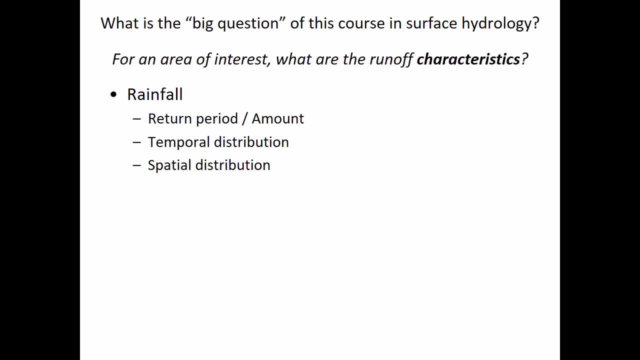 to be a very intense rainstorm all at once, like a thunderstorm, Or is it going to be like a long low-intensity, drawn-out storm that maybe doesn't cause as much runoff at a peak time? Spatial distribution is talking about. 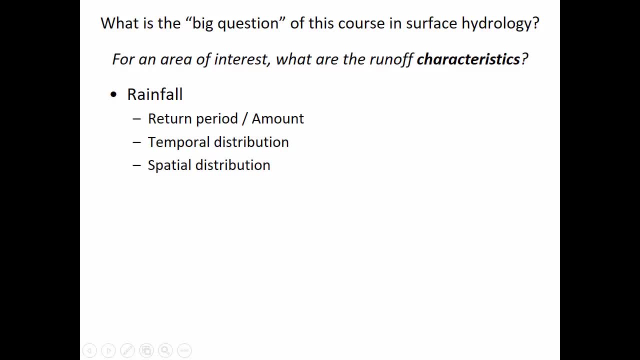 How is the rainfall variable over space? It may rain a lot at the airport, but does that mean it's going to rain the same amount in Huntington, when we're X miles apart, Or are there certain features in the environment where it consistently rains more than others? 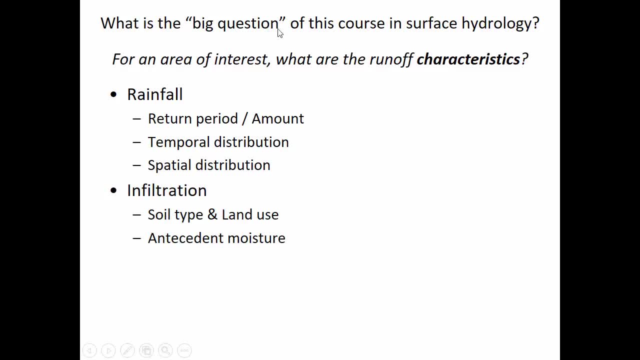 So we'll look at all of these. when we discuss rainfall, The hydrologist has to characterize infiltration, And so the hydrologist needs to understand the characteristics of the soil and also what's on top of the soil. You may have a. 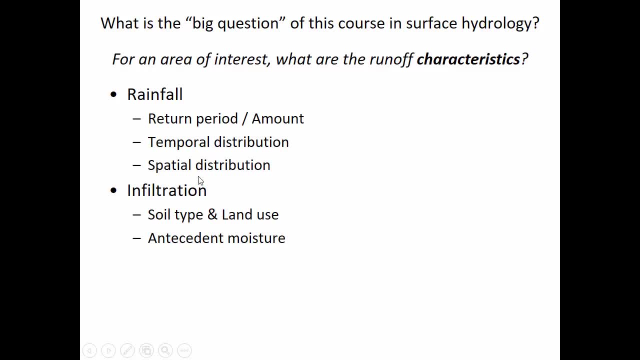 really well-drained gravel and sandy soil, but if there is pavement on top of it, then there's not going to be very much infiltration. Or you may have a really nice grassy field that's not too steep and you'd think, wow, a grass can infiltrate water really well. 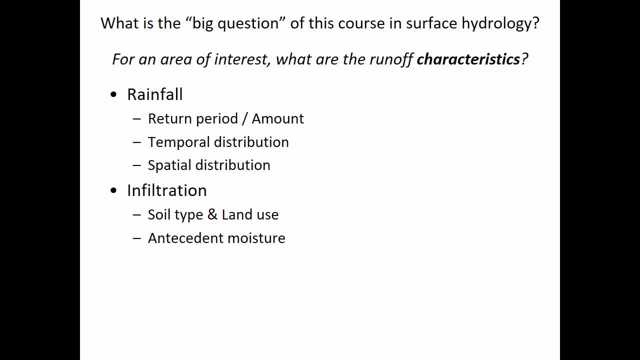 But if there's clay soil underneath it, like at my yard- my house has a lot of clay soil- it's not going to be infiltrated. So it's not going to be infiltrated. But if there's clay soil underneath it- like at my yard- my house has a lot of clay soil- it's going. to be infiltrated. So it's not going to be infiltrated. but if there's clay soil underneath it, like at my yard- my house has a lot of clay soil- it's not going to be infiltrated. But if there's clay soil underneath it, like at my yard, my house has a lot of clay soil. 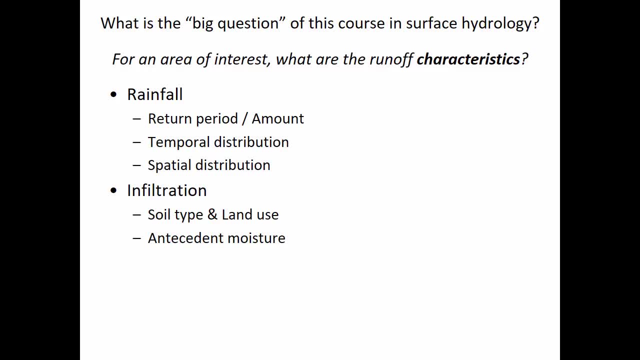 it's going to be infiltrated, But if there's clay soil underneath it, like at my yard, my house, is like all clay everywhere- It does not absorb rain and it becomes very squishy, And so that's one of the things that a hydrologist has to understand- is the soil characteristics. 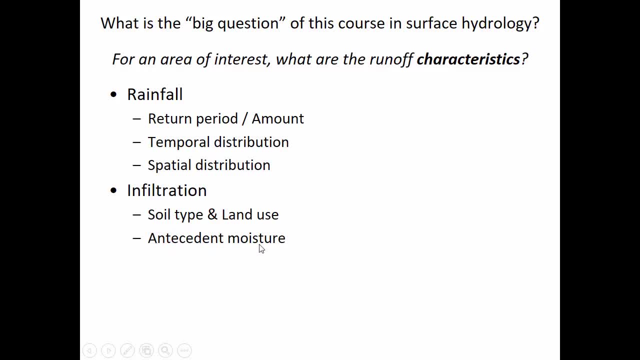 and land use, And also this word antecedent moisture just means: is the water already saturating the soil from a previous storm? And so you have to make assumptions or have data that describes, prior to your design event. You know the thing that you're planning for. you have to decide how often is your system going to fail? 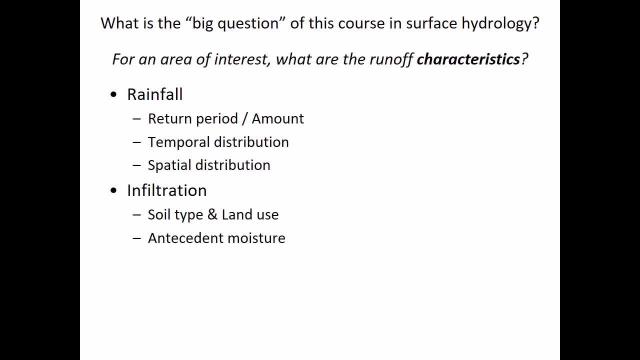 It's always going to fail eventually. The question is: do you want your system to fail once every 100 years, once every 50 years, every single year? You have different standards for different type of roads, for example, And part of that goes into the assumptions- is how rainy it was before your design event. 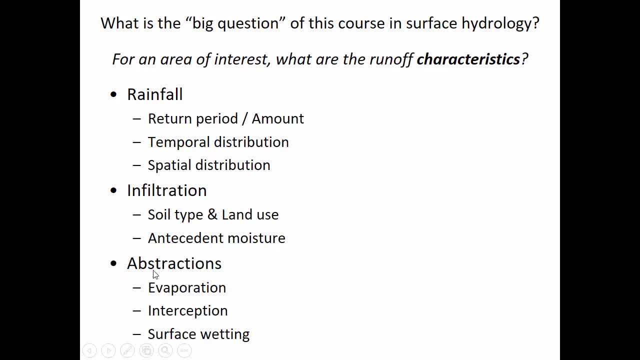 There are these things that are called abstractions, And what the abstractions do is they either reduce or delay the amount of water that runs off. So things like puddles or ponds, evaporation interception by buildings, the wetting of a surface, 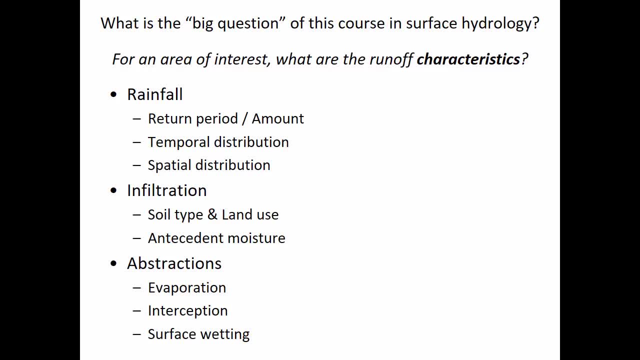 Before the water starts to flow, the asphalt has to get wet, And so there are these things that we have to make Assumptions about and study so that we know a little bit more about the timing of when the peak is going to arrive. 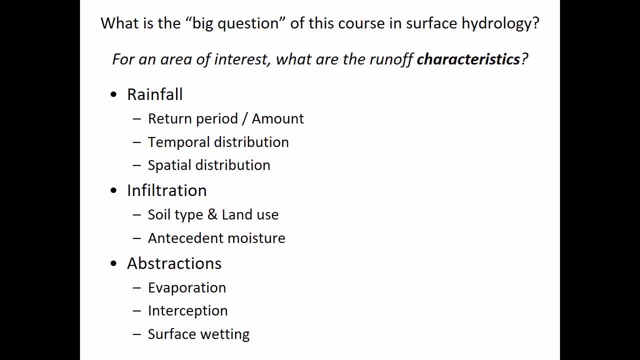 You've maybe noticed before that when the rain starts it's still dry underneath the tree right, And it stays dry under the tree for kind of a long time. all things considered, You'd expect, maybe, that the water would just immediately run off the leaf. 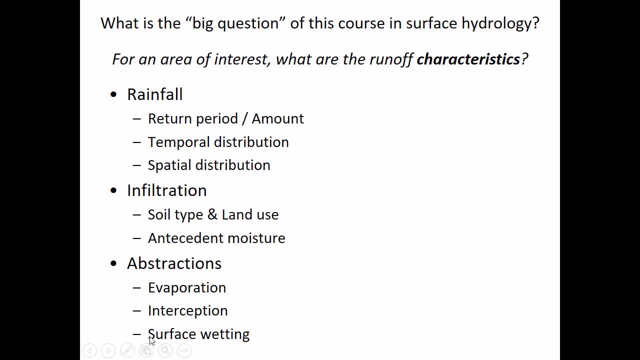 But the abstraction of vegetative interception can have a huge effect, And so we study those sorts of things And there have been empirical evaluations done of different types of vegetation and how much of an abstraction they have. Now this is all theory, And this next column is mostly practice-oriented. 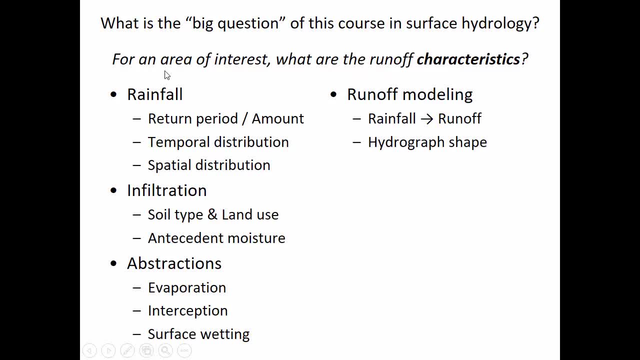 And so we have to understand, like the fundamental forces of how water is moving around and really what's happening. But it's also complicated that there's no, There's no fundamental way that we could say: you know an individual molecule of rain that's falling through the sky, where that molecule is going to end up. 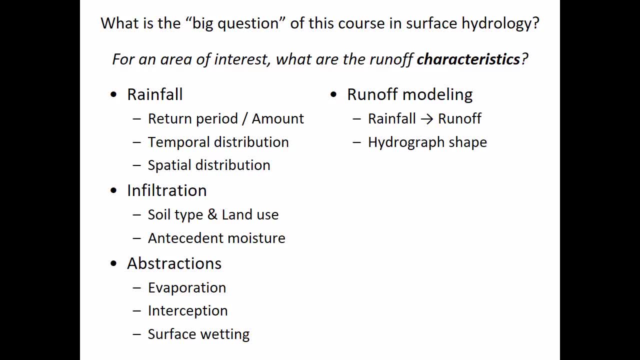 So we just have to use shortcuts to do that, And so we have to come up with approaches that describe the relationship between a certain amount and timing of rainfall with a certain amount and timing of runoff. There is a graph, It's called a hydrograph. 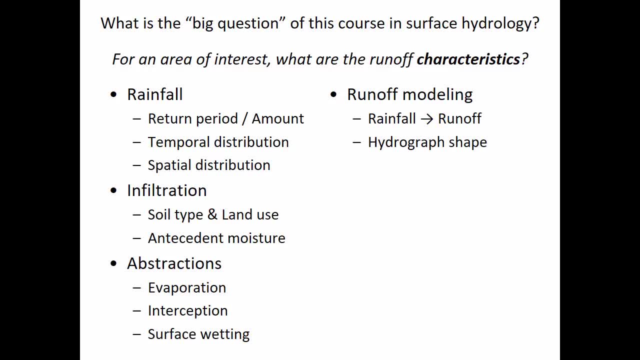 That is time versus flow rate Q And what we're often interested in. across the top of this then we would maybe represent rainfall amount And so, like this scale is rain, And so it was a little bit of rain, and then it was a lot of rain, and then it was even less rain. 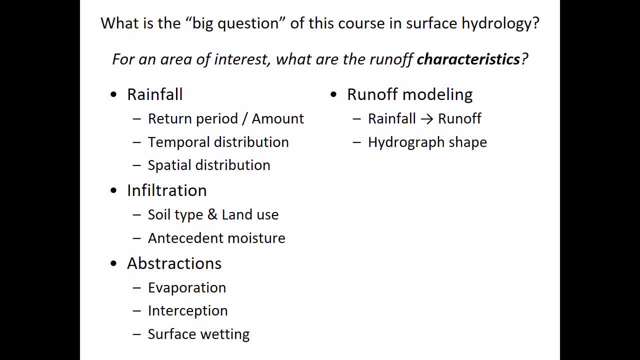 So this is called a hyetograph, And it's really important to know how long of a delay between when it rains and when the peak arrives, And so there's all these different methods that have been developed over the years in different places to try and understand what's the relationship and the delay. 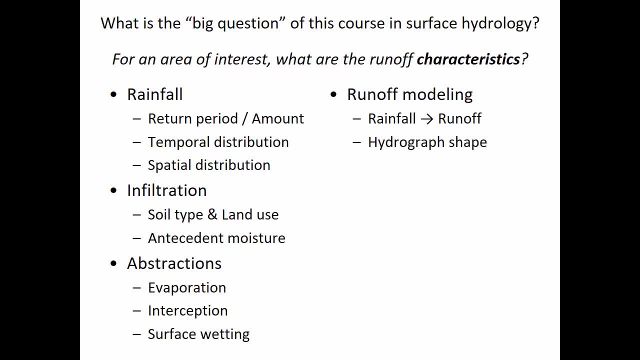 So now, if we take a look at this graph, it's hassle-free, And the problem we've come up with is a bit of a delay between when it started raining and when the creek rises. It's not instantaneous, But the steeper the watershed, the more quickly that peak wave arrives. 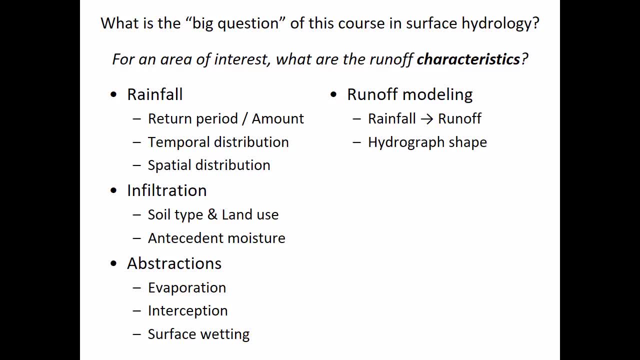 The more rocky and previously saturated the soil is, the more quickly that wave will arrive, And the shorter the time between the rain and the runoff also increases the amount. So there's a real extra-total delay between when it started raining and when the creek rises. 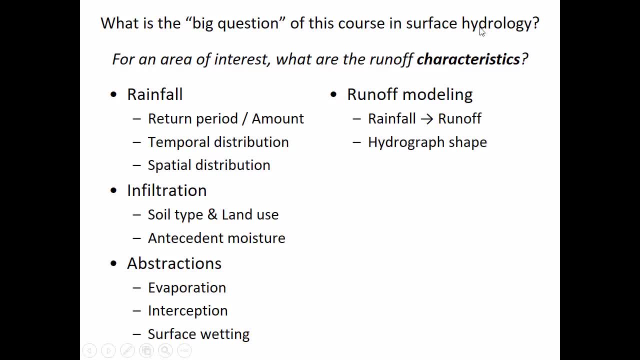 There's a relationship between the delay and the quantity, and so there's a lot of different techniques that have been developed over the years that allow us to understand this relationship between how much and when of the rainfall versus the runoff. Any questions? so far as we're just taking this top level view of the concepts, 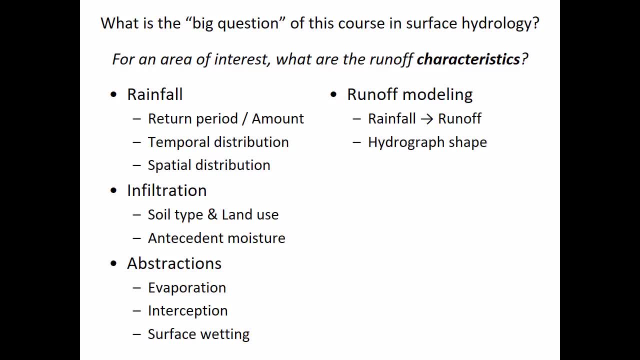 I'd encourage you to occasionally, by the way, look back over this list that we're developing, because we're going to be getting deep into the weeds on things that just seem so obscure, like why does water evaporate. You'll be wondering: why are we talking about evaporation of water for a whole class period? 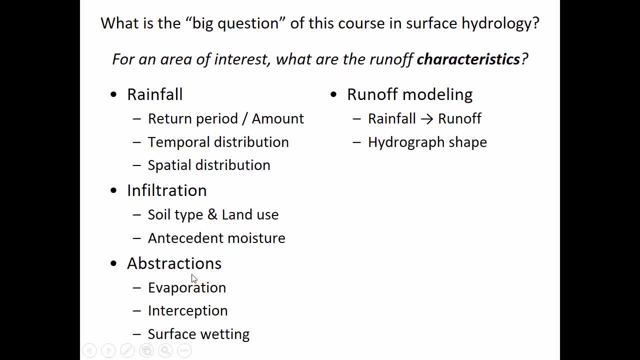 It's because we want to know about the abstractions and the things that reduce the amount of water that's getting to the runoff. This is kind of like the time that we're going to look at it all at once. Routing is the idea that there's a delay once the water gets to the creek. now the 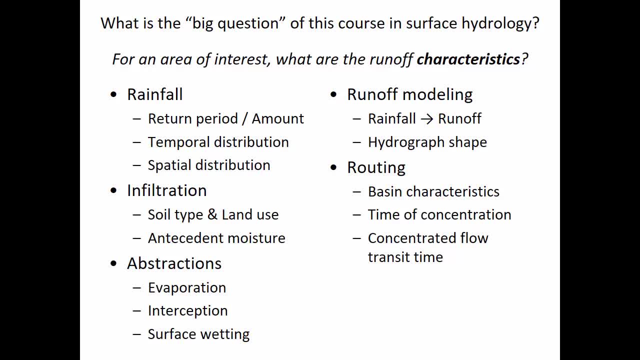 water is traveling down the creek. There's a travel time of just the water flowing through the river and as the water is flowing through the river, the water at the bottom of the creek is moving slowly and the water at the top of the creek is moving fast. 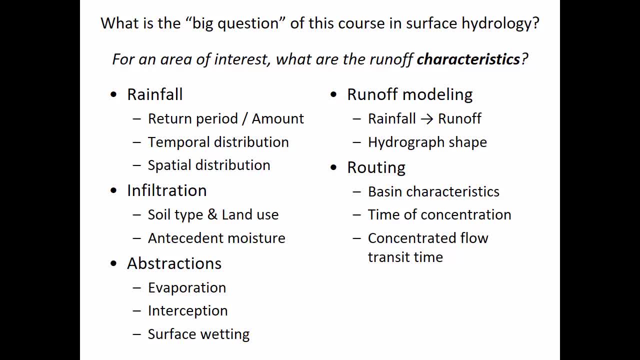 Does everybody remember, Remember the idea of a velocity profile? You remember what we said is like: okay, so this is depth and this is velocity, So the shallow depth water isn't moving very fast, but the further away you get from the 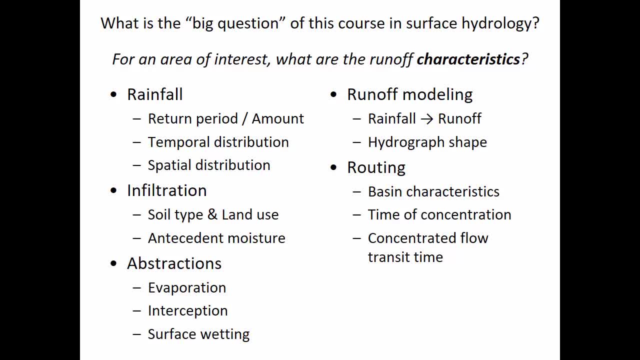 bottom of the creek, the faster it's moving. Everybody remembers the no-slip condition from fluid mechanics and the idea of a velocity profile. So, as the water, So it's going to be like a big surge of water, like, if you think of it, like a bucket of water. 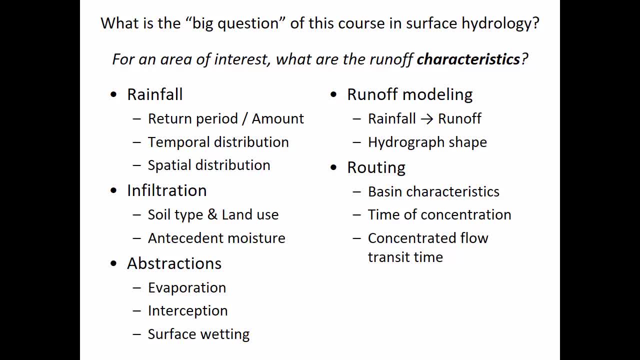 got poured into the creek. Well, if you can pour that entire bucket of water into the creek all at once a mile down the creek, it's not going to arrive in the same amount of time it took you to pour it out of the bucket. 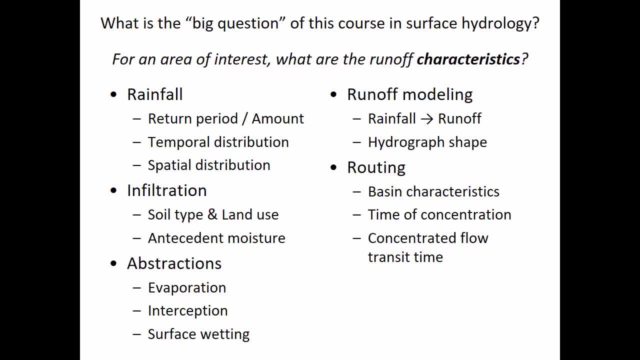 If you poured it out of the bucket in five seconds. it's not like a mile downstream. suddenly a big surge of water just arrives and it all arrives within that same five second window. It's spreading out because the stuff at the bottom is moving slowly. 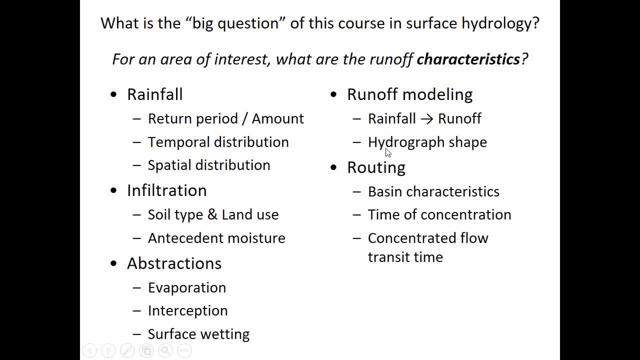 stuff at the top is moving quickly, and so that effect is the routing effect. it's travel time and delay, and so routing can be used to talk about hydraulic routing, which is the flow through the channel once it's already concentrated. but routing can also include analysis of shallow water flowing. 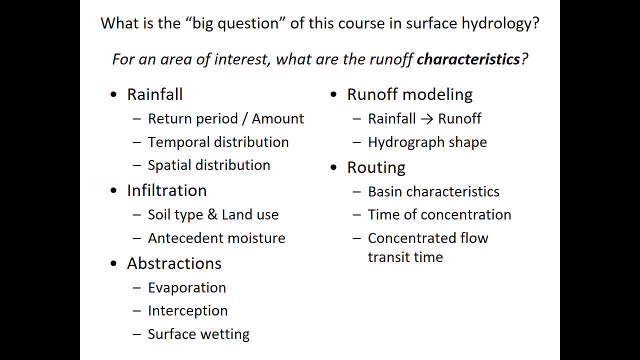 as a sheet over the surface of the land, and so it's aspects of delay time that that are really important in saying to the hydro, the hydraulic engineer- remember the hydraulic engineer. she wants to know what is q to size the pipe, and so we have to account for all of the factors that are. 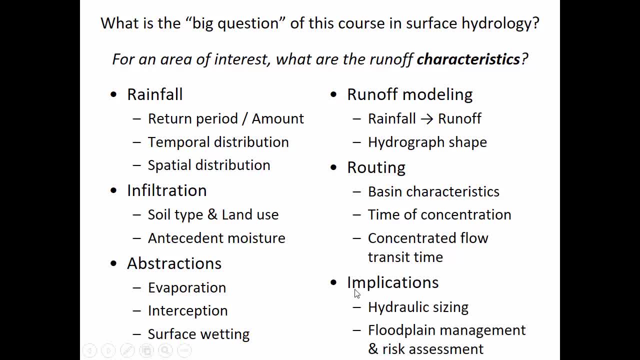 going to cause that flow rate. finally, the the implications of all this we're going to study this semester is pipe sizing and then also flooding. you know communities that are adjacent to creeks and if you think about west virginia, like, what community is not adjacent to some sort of a creek or a river? i honestly can't think of one. 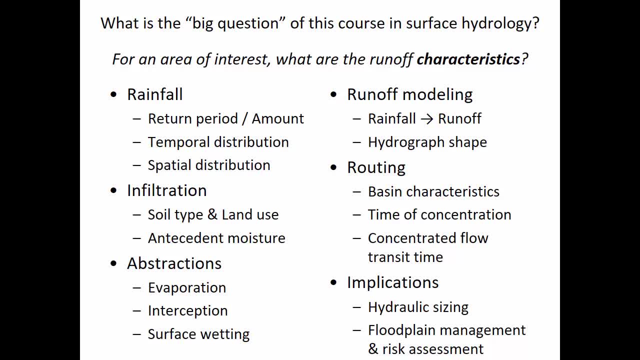 i mean, and the reason why is that that's really oftentimes the only flat land is next to the creek, and so people are in the habit of: well, i don't have to do the earthwork here, because it's already flat, so i'm going to just park my house next to this creek and then you're in a lot of risk, you're. 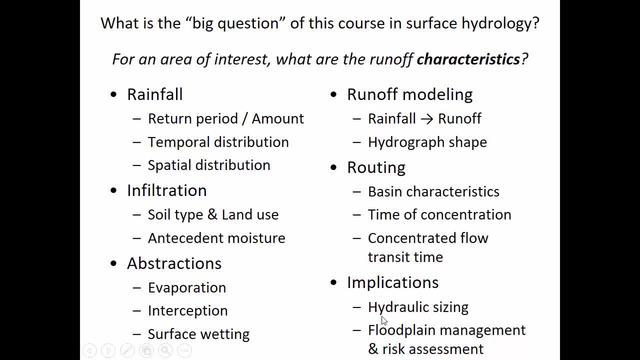 at risk of flooding, and so towards the end of the semester we're going to combine hydrology and then the floodplain management, and then the economy, and then we're going to go to the borderline with the floodplain management. we're going to be doing a little bit of 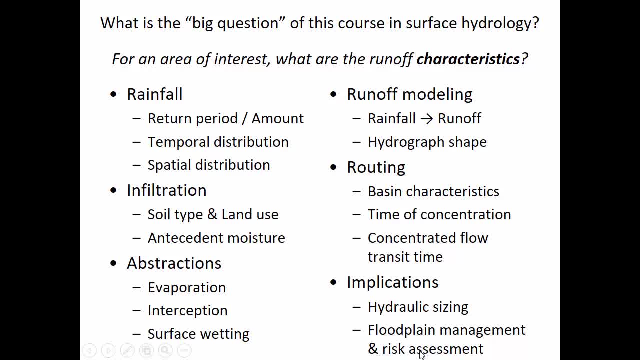 saving economics and look at certain things we can do to reduce, reduce the risk of flooding and compare the value of those measures to the cost of those measures. and so we'll do a little bit of statistics, economics combined with the hydrology, with the risk assessment and floodplain. 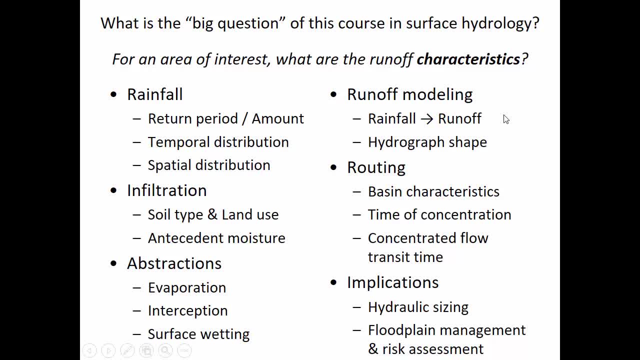 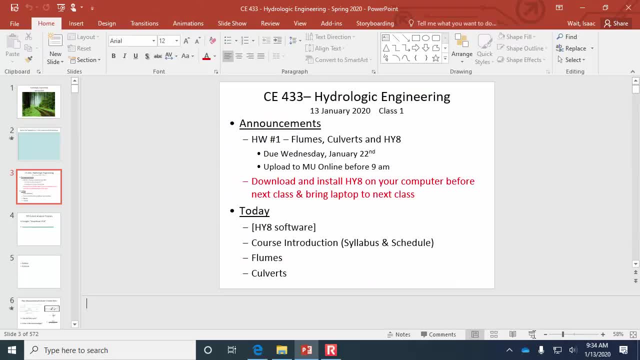 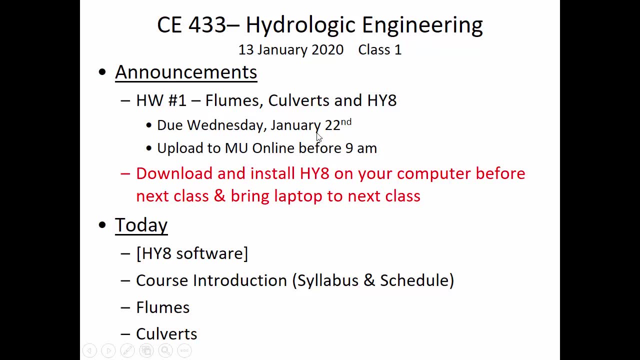 management. so this is what we're doing this semester. Well, that leaves us hold on a minute. Yeah, okay, So here's today's announcement slide. The Flume, Culverts and HY8 assignment is due Wednesday of next week. It's available now for you to look at on Blackboard. 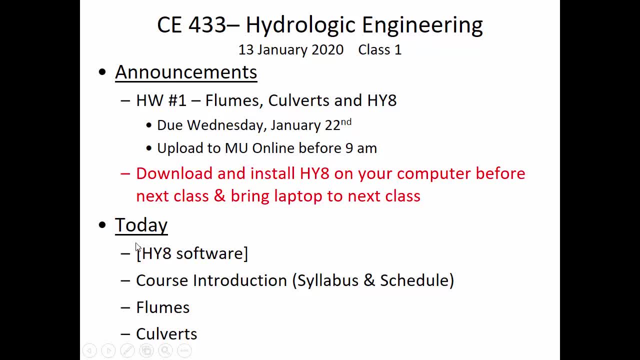 You need to download and install the HY8 software and bring it to class, bring your laptop to class on Wednesday. On Wednesday, I'm going to be demonstrating how to use HY8, and then on Friday you're going to be using it to solve a couple of example problems. 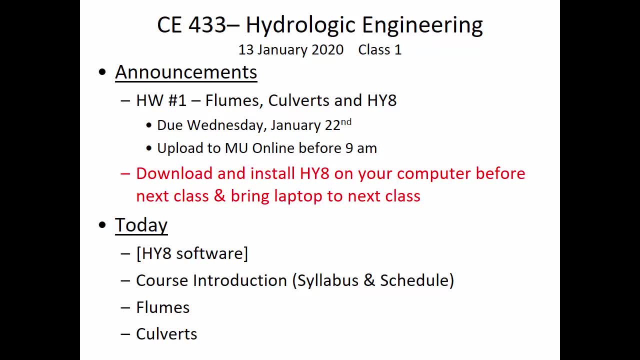 You may get a chance to actually use it also on Wednesday, but at the very least I'd like you to have it installed so that you can follow along with the problem that I'm solving. Yes, Jeffrey, So on the schedule here, if there's like a mark after a lecture, does that mean you're continuing on from the few days left today? 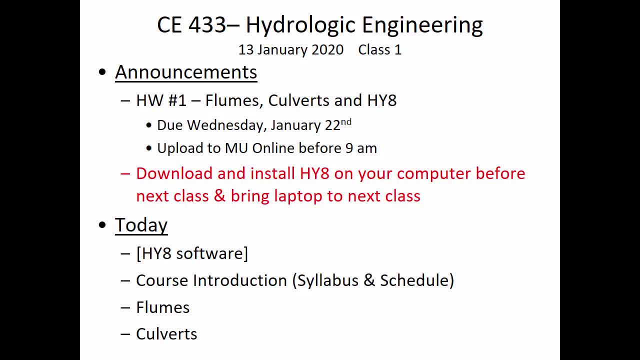 That's right, yeah, Yeah, so Friday, for instance, we're also doing HY8.. Okay, I was trying to figure it out, Mm-hmm. Yep, And on the schedule you can see the corresponding textbook chapters, and that textbook chapter information can give you an idea of which terms you should learn. 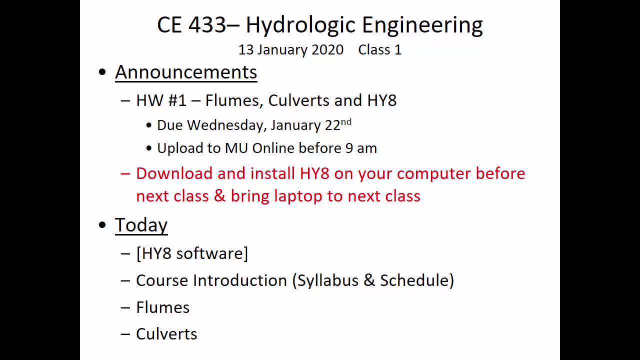 You know rather than learning all the terms. you can learn all the terms You know rather than learning all those terms at one time in the semester. maybe it'd be best to start with, like the Chapter 16 terms when we're talking about that and go roughly in the order that we're learning it. 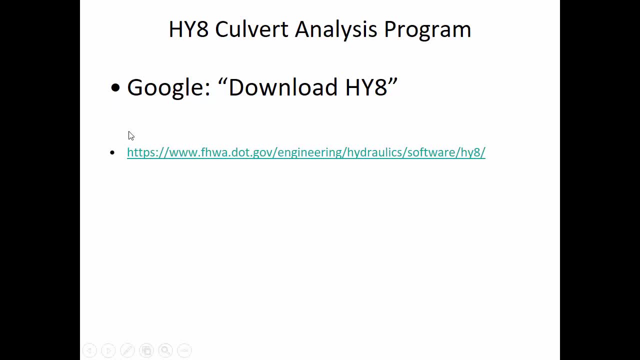 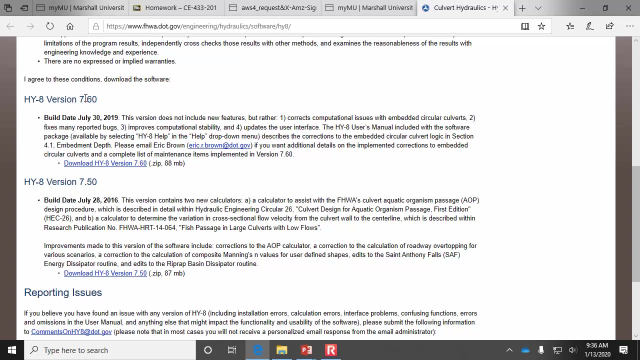 All right, Here's what it looks like when you just Google the phrase download HY8.. The top hit is going to be a link to the Federal Highways Administration And just right there There, HY8 version 7.60.. And you just click download. It's archived. It's a zip file, but once you decompress it, the installation is in there and it's fast, It's easy. 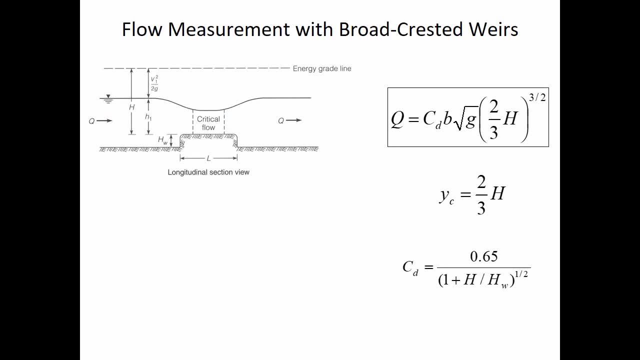 Okay, weirs In hydraulics. weirs are used to measure flow, And one of the things that we can do to measure flow in an open channel is just put in an obstruction, Like if it's a concrete channel. you know water's flowing downstream in a manufactured, engineered concrete channel. 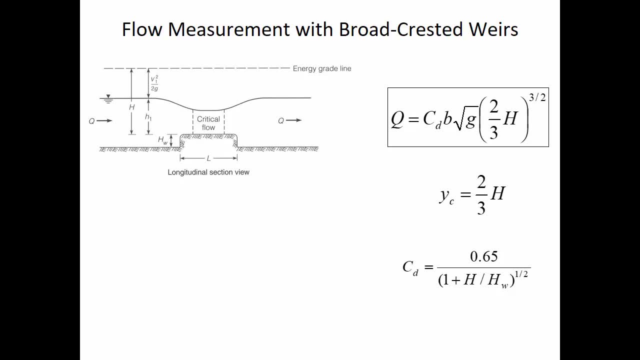 If we put a big step in the middle of that channel- and it's big enough, what it will force to happen is critical flow over that step, where the surface of the water will actually dip down and flow at this special depth. That's like a concave slide, and then the water flows down to the central channel. 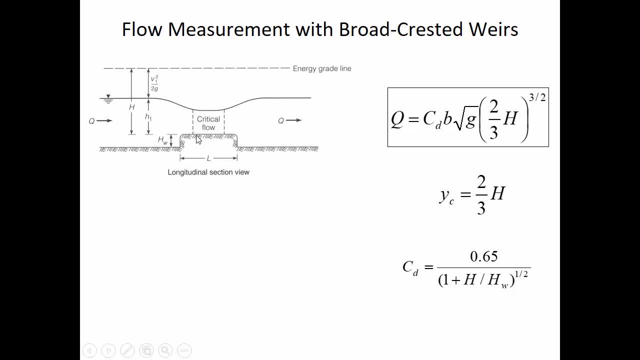 That's like a concave slide and then the water flows down to the central channel flow at this special depth and if we know it's doing that, we can quantify the flow rate with the weir. so that's the, the summary, or the real quick. 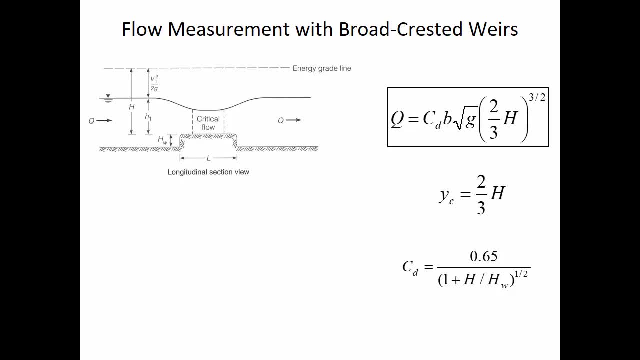 introduction to what a weir is doing is. you'd use it to measure how much water is going through the channel, and so the disadvantage of a broad crested weir like this is that this step tends to accumulate trash. debris like sediment or logs or whatever gets in. the creek is going to accumulate behind this weir, and 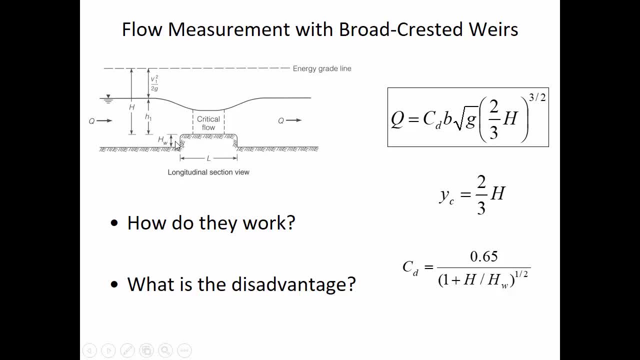 the other thing is that you lose some energy, like it can obstruct the flow and the water depth can get deeper upstream because you've put in this, this step that the water has to flow over. well, it can cause choking upstream and so there's some disadvantages with a broad crested weir. this is a side view of it. 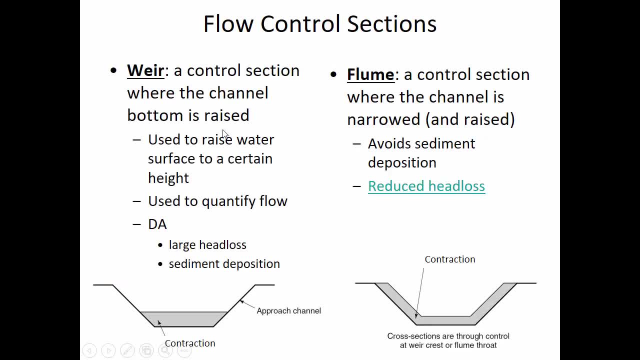 instead of using a weir, there's another way to quantify flumes that eliminate some of those disadvantages. and a flume. rather than having the channel contract from the bottom up, like the step that the water has to flow over in a flume, what we're doing is we're making a channel temporarily narrower and so by forcing 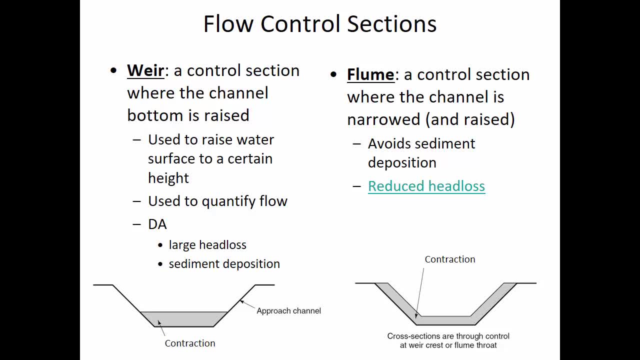 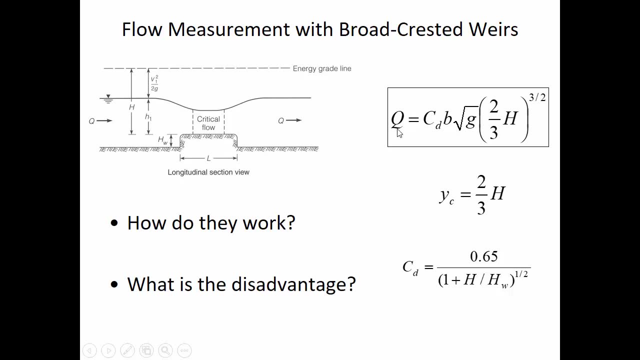 the water to flow through a narrow channel. we're doing the same kind of thing where what we're going to do is create a relationship between depth and flow rate. graphically. we're going to determine that walked it to be a reference point for using an energy grade line- vibrational- and so what we're going to do 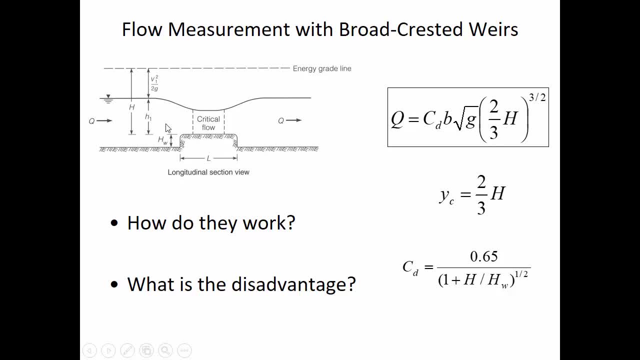 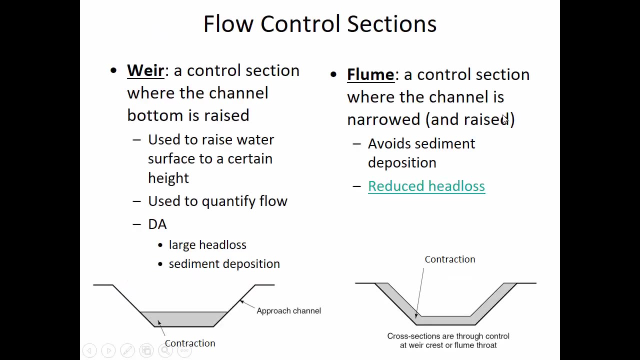 is we're going to thicker up a profile product. so if I measure up depth in flow rate, which is in terms of the operation vehicle phase approach, and we can have an equation with the weir that says- I just show you that equation here- q as a function of H, and so H is the depth from the energy grade line down to the height. 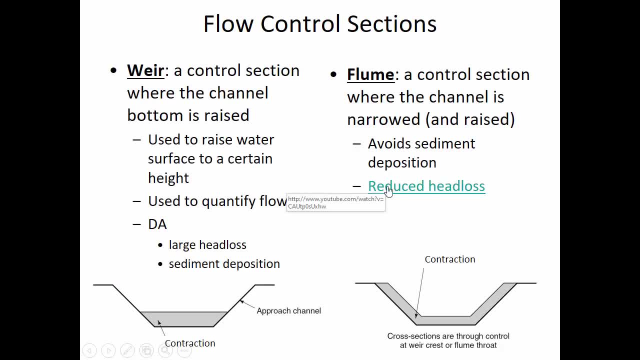 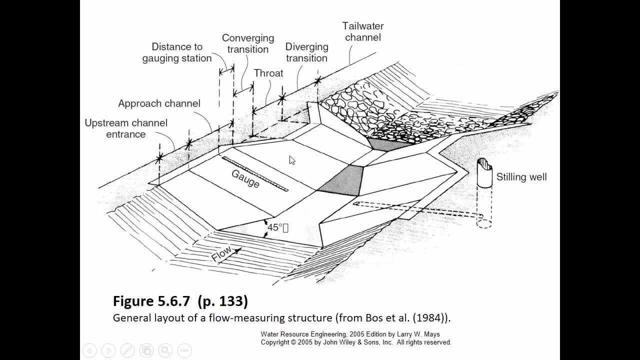 deposition, and it doesn't cause energy loss or choking upstream, and so the reason why it avoids sediment deposition is- this is kind of now an angled view- I've got a side view in just a minute- but the advantages is that actually the water speeds up as it goes through the flume and so it scours any sediment that. 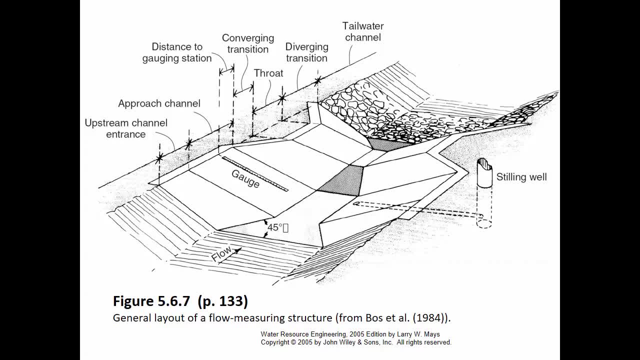 would have settled, instead of slowing down like it does upstream of a broad crested where a flume accelerates the flow, and so there isn't going to be settling of the sediment. and what we do you'll notice here where it says gauge- you, measure the water depth before the water goes through a contracting section. 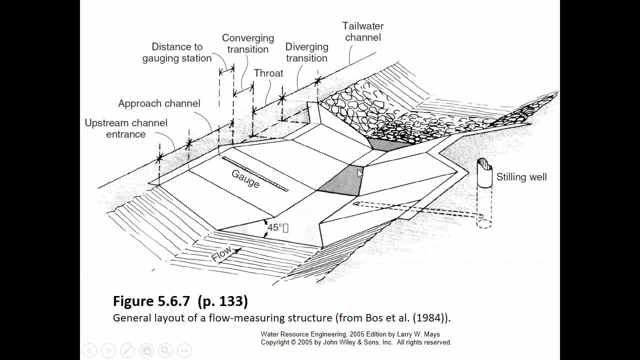 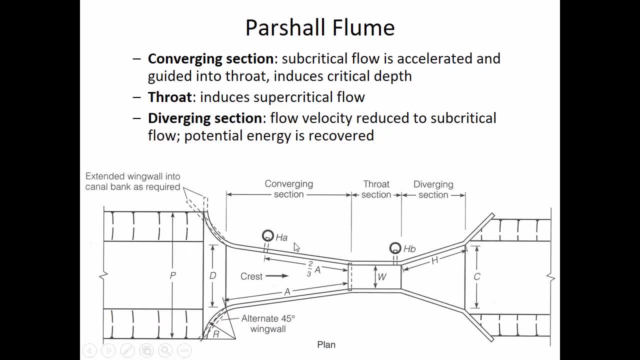 and then down a slope, you can't quite see the elevations. let me move on to this view. this is from the top and what it shows is that the chance that the water is going to precipitate on a slope is going to be. channel is getting narrower and we're measuring the water depth before it gets to a throat. 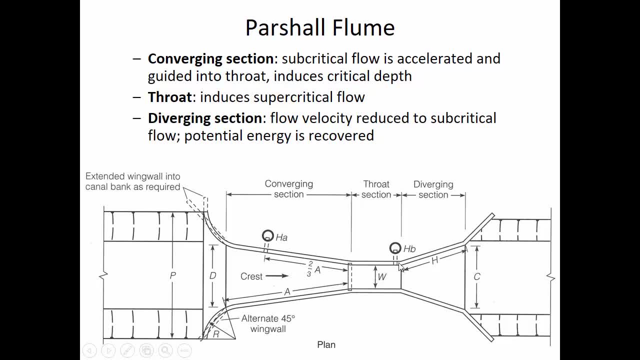 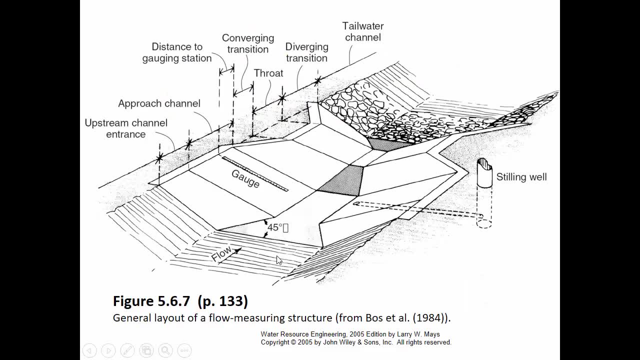 The throat is where there's a really steep downhill section. We also measure the depth in the throat for a reason I'll explain in just a minute. Let me go back now to the side view of this flume. You can kind of tell here in the approach and then in the throat it's 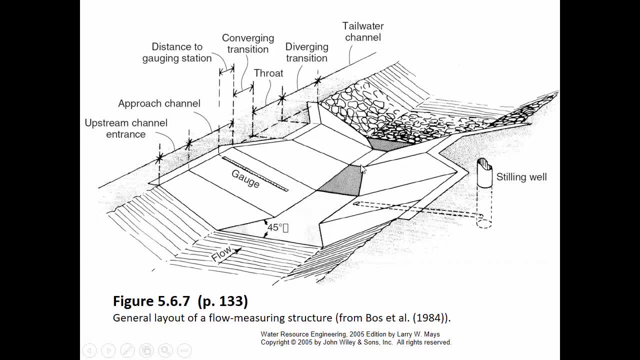 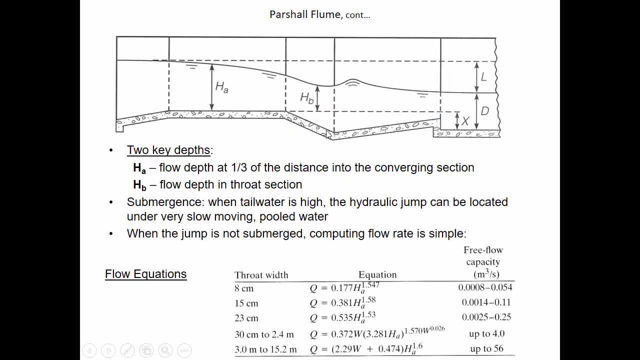 going downstream, and here's the side view that shows it a little bit better. So we're measuring the depth before the water goes down, and in the downhill section, in the throat, we're also measuring the depth there. Now we're doing the same kind of thing where we're 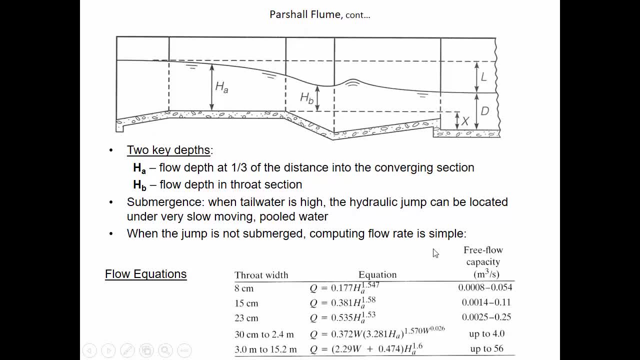 using this to predict what is the flow rate. Think about a farmer and the farmer is drawing water from an irrigation canal and sending that water out into fields. 007, 008. The farmer. maybe, if you're in the western United States, there's limits on how much water can be. 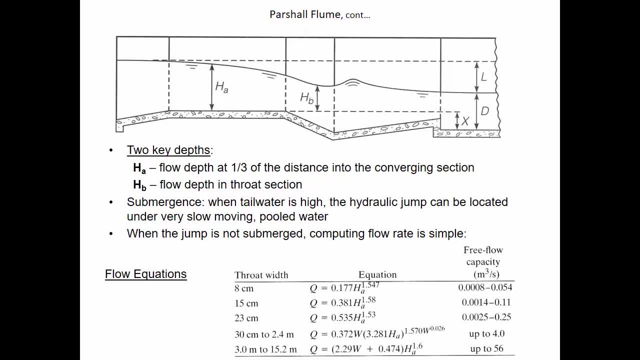 extracted, They have what are called water rights, and so a farmer is allowed to use a certain amount of water each day, and there isn't an instrument like an electronic gadget that says how much you're taking out of the creek. If there's a pump, of course, you can quantify the flow rate that way. 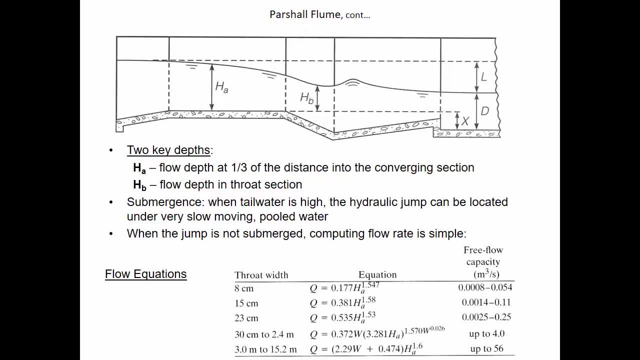 but in open channel flow it's a little bit more tricky to know what's the flow rate. So what this Parschall flume would allow the farmer to do is you'd set up. it can be even plastic, or they may have a concrete flume that they send the water through before it goes into their fields. 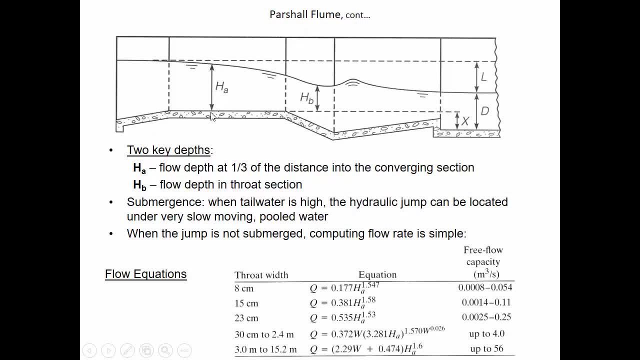 They would measure the depth of flow, H sub A, that's the height of the water at location A, and then you'd plug it into these empirical equations that manufacturers of flumes have come up with. There are these standard designs that have been out there for a long time, and 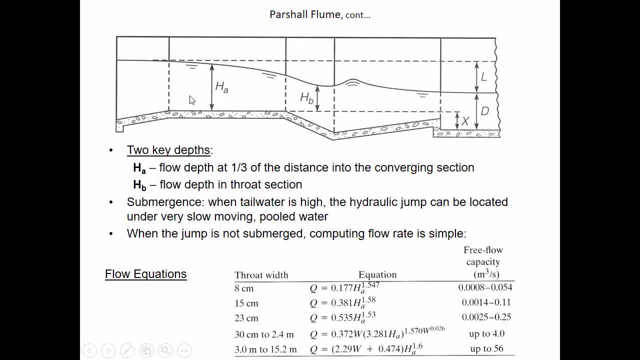 they've calibrated to know, for a certain depth of flow, what is going to be the flow rate 009, 008. the flow rate Q going through a flume. Now, the tricky thing about a flume is if there's a lot of water down stream. Let's say that you've put the flume into a creek. that's pretty shallow. 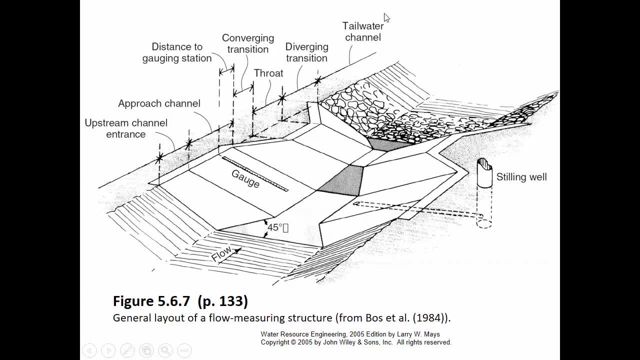 and the tail water is just talking about where the water goes after it comes out of the flume. it just Não means you could add water: 216, 008 meterHA, 202, subjectivewhat's the most common form I had heard already because I needed to ink anything over there. but yesterday had happened before me so I thought I'd go ahead and put the water over there. You can't put it there, So what? 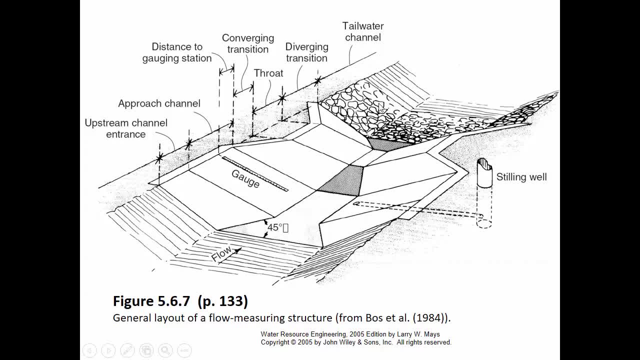 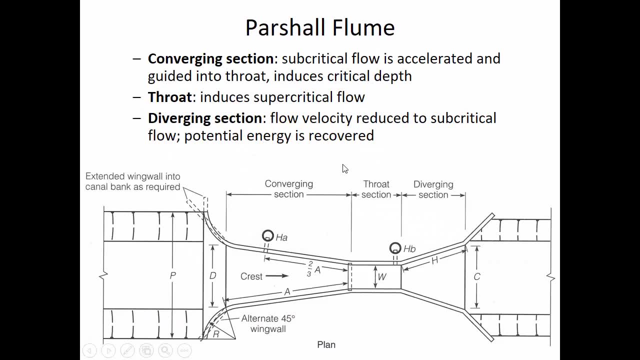 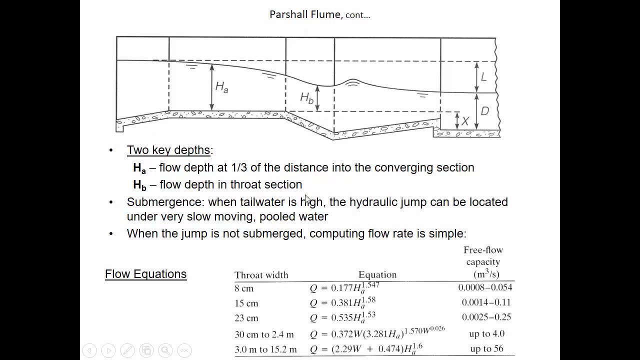 of the flume. If the tailwater has a pretty high depth, then the hydraulic jump that forms inside of the flume is going to be submerged, And so these equations that are right here are called free flow equations. They assume that this hydraulic jump that's occurring 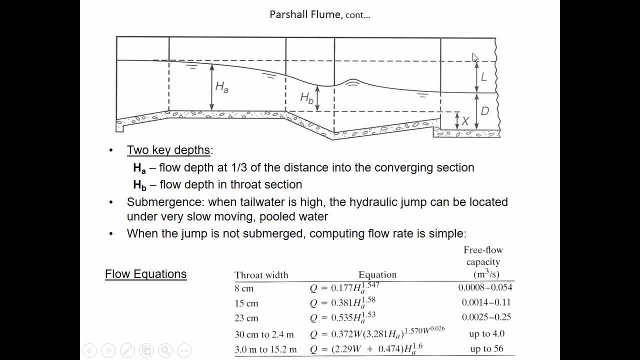 isn't choked by the tailwater, But sometimes, if the capacity of the channel downstream is kind of poor and the water level is high downstream, then that can cause the hydraulic jump that's occurring inside of this throat to be drowned, And so you just have to apply. 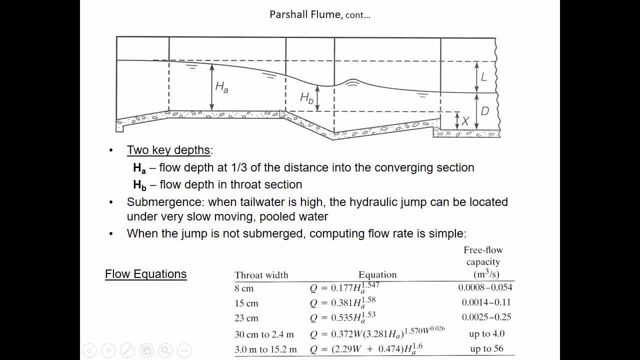 a correction is all it is. You look at, you're measuring the depth in two locations and if B is really high compared to A, that tells you I'm going to still use this equation, but then I'm going to apply a correction factor Because B being so high, it's going to be. 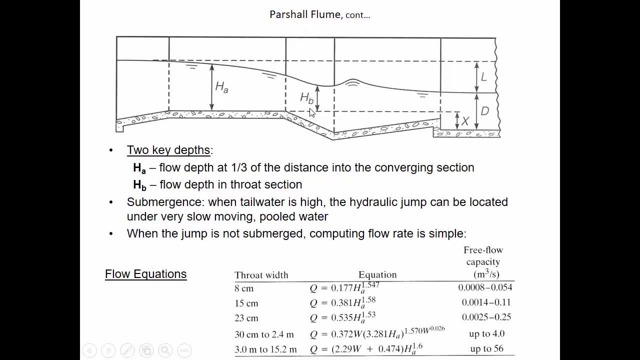 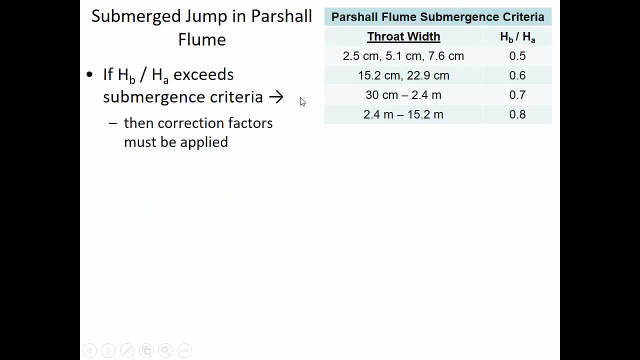 reduced the capacity through the flume, So what we're going to do to get a feel for that is we're going to work through a problem. We're not going to do it today, though, because I don't want us to rush through it and make it an afterthought, But let me just walk you. 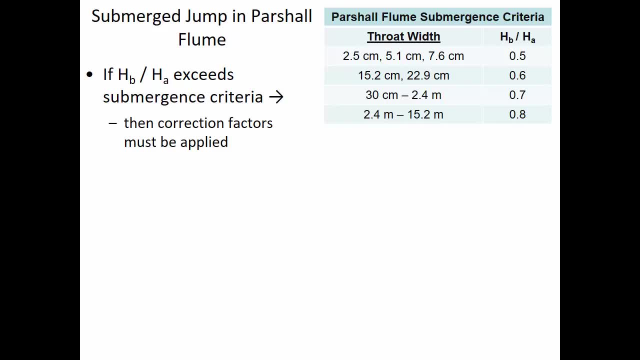 through the process so that we can jump right into the example problem when we get together on Wednesday. You're looking at the ratio of B- the downstream depth in the throat- to the depth A, Which is the depth in the converging section. So we kind of want to look like what's the 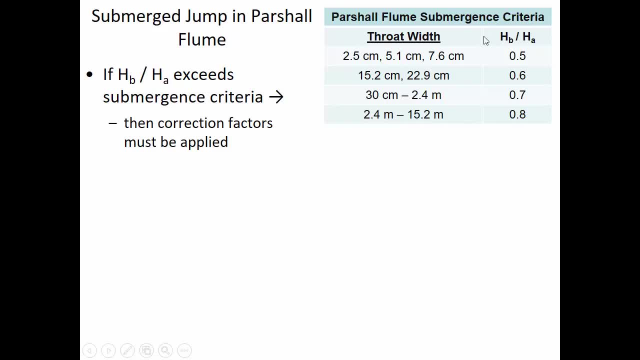 ratio of depth, And this is a limit. If you are above this limit, then that tells you you have to apply a correction factor. So if B is, for instance, in a 30 centimeter width throat, if the depth downstream is 70 percent as high as the depth upstream, then 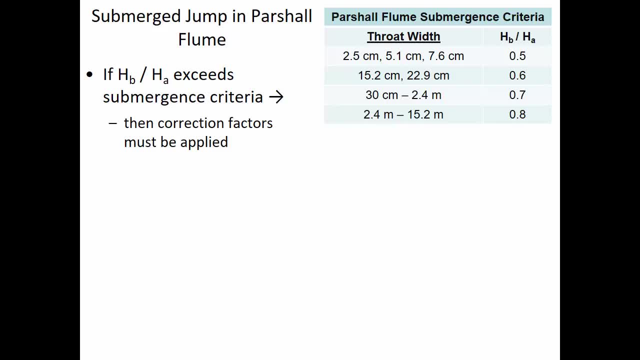 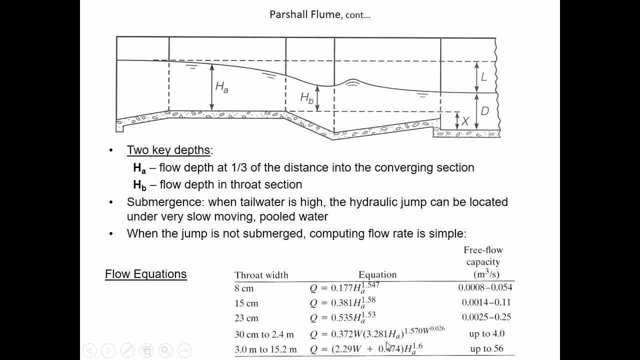 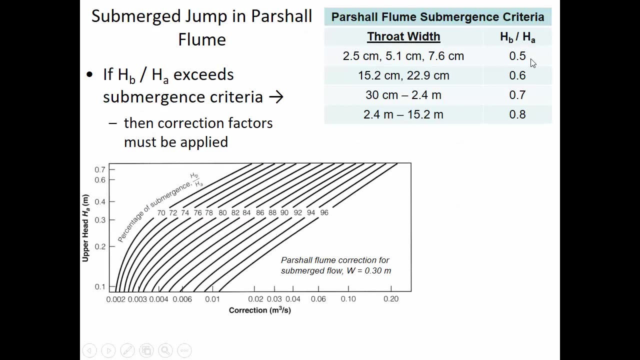 beyond that you'd have to apply a correction factor. Below that you don't have to apply the correction factor. You can just use the free flow equation that we had to begin with, this original equation. But if B is higher than the criteria limit, then you have to. 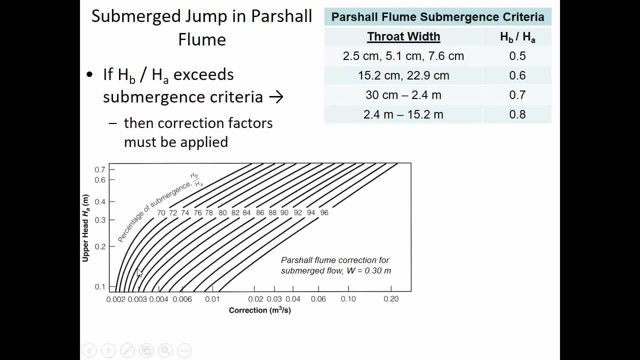 correct And the way that you correct is with a figure like this. Now, this is a figure that's specifically put together for a throat width of 30 centimeters and there's curves like this for a whole variety of other throat widths. So if you are below this limit, then you would have to apply a correction factor Below that. 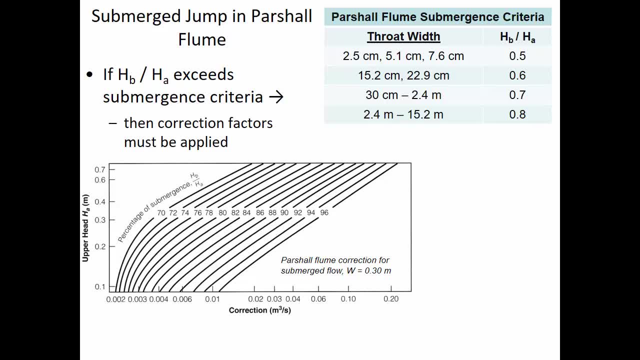 you would have to apply a correction factor. Below that, you would have to apply a correction factor. All right, so you can see that the denatured growth is falling off. It's fine too. And then we have to add a function factor. Up to this point, we're just going to look. 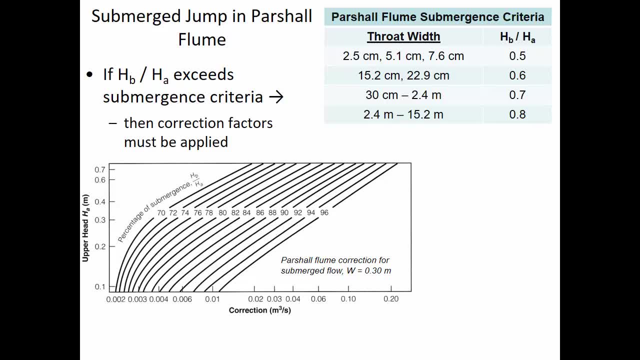 to the line we're looking for. So the line we just drew or we're setting in this equation would be equal to the denatured growth. they probably have a section where they're selling these partial flumes. by the way, partial was the name of a guy, it's not partial spelled incorrectly. 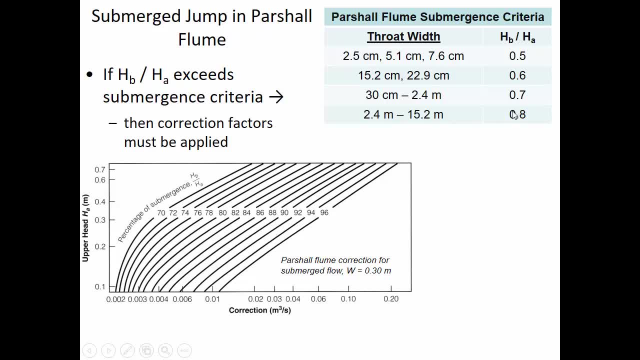 that was a person. so what you do is if the, the downstream depth in the throat is too high, then you'd correct and you'd look up like what is your specific B to a ratio, and so you'd find like what percent submergence is there? and then 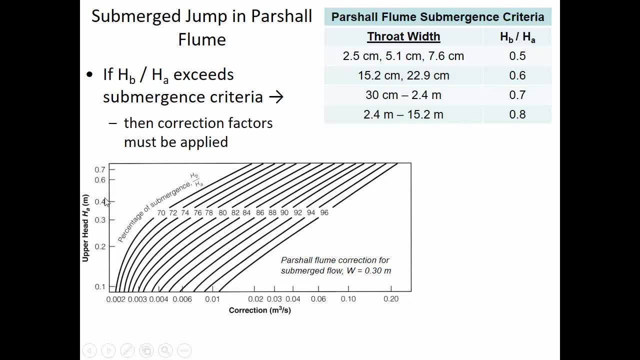 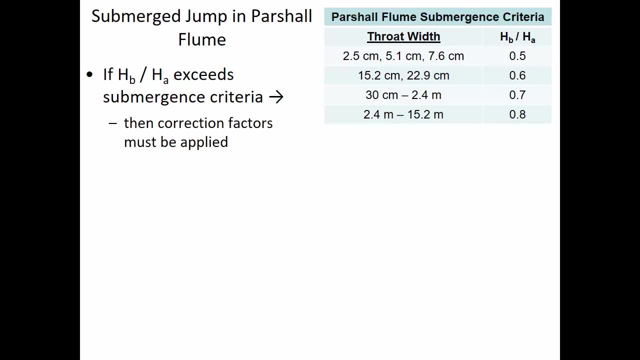 you'd find out what is the upper head. so if you had measured an upper head of 0.3 meters and it was 80% submerged, then you'd go down and find what is your correction volume like. how much of the flow rate do you need to subtract off of? 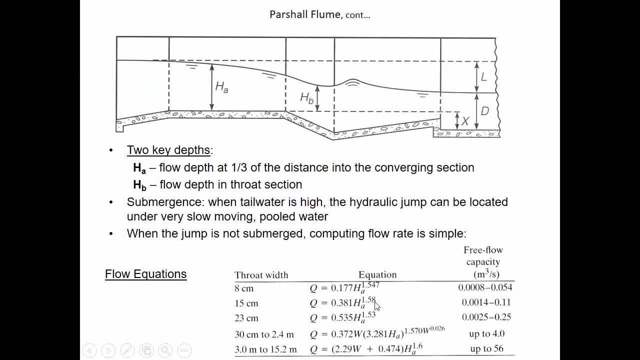 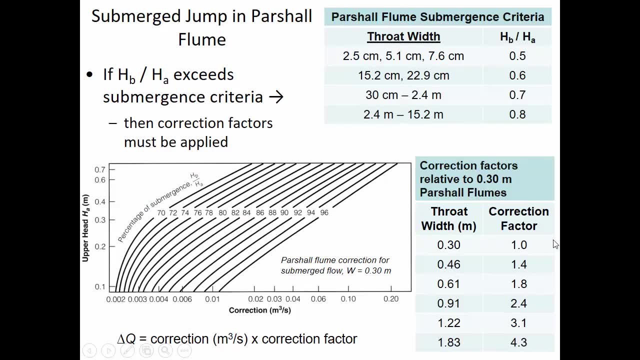 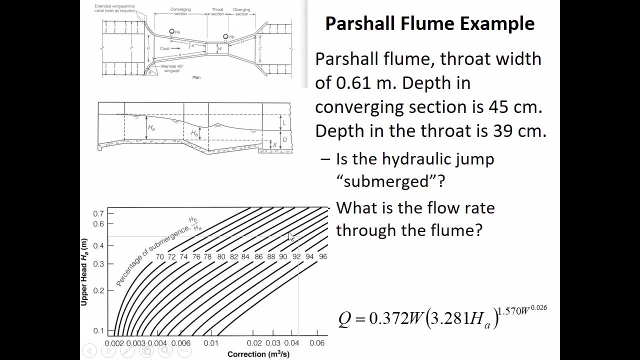 what the equation itself gives you. so that's what we're going to work through. we're going to go through that process in class, and I'll also explain this correction factor in a different way. we're going to work through this example first thing on Wednesday. so what? 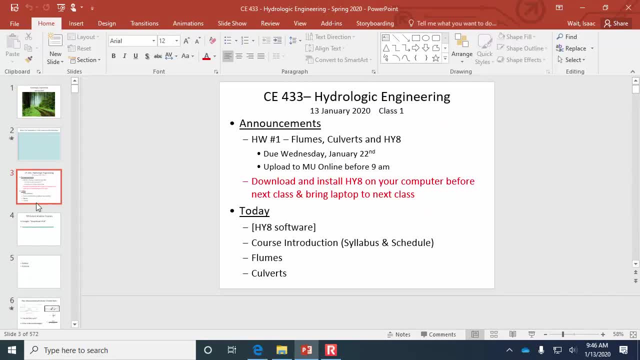 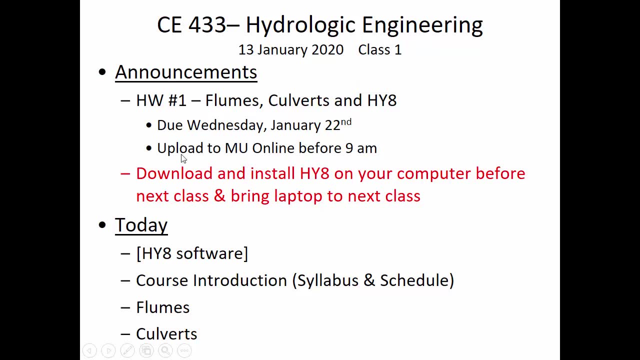 should you do? let's just go to these announcements. the the homework isn't going to make a lot of sense yet, but it will as of Wednesday. so I think really what you need to focus on is, if you don't already have the textbook, I'd encourage you to get that. the textbook is.